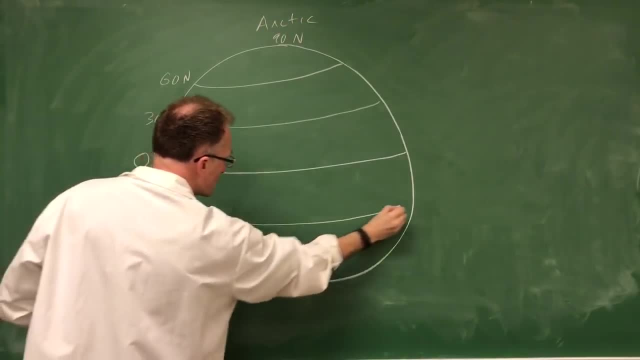 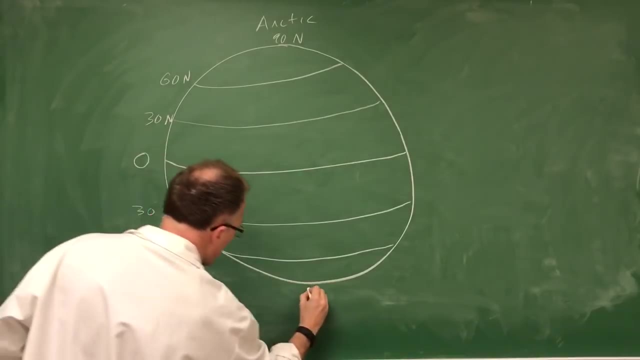 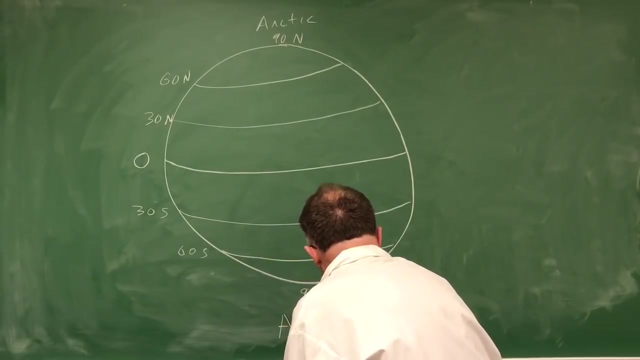 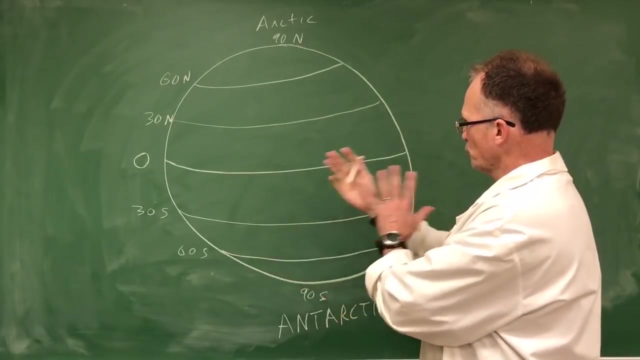 And let's go down the other way. So this is 30 south, 60 degrees south, and this is 90 south. So this is Antarctica. Okay, so this is the basic geometry. Which way is the Earth spinning? Spinning on its axes? We know that it's got to be spinning this. 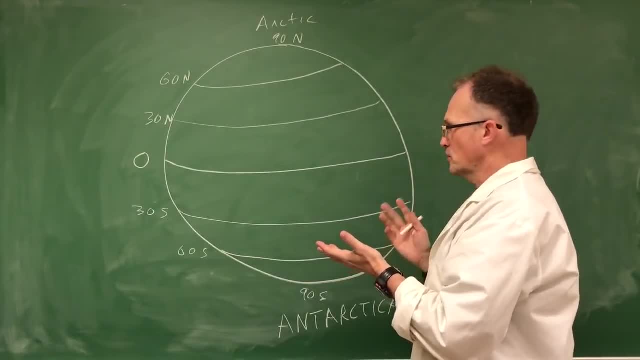 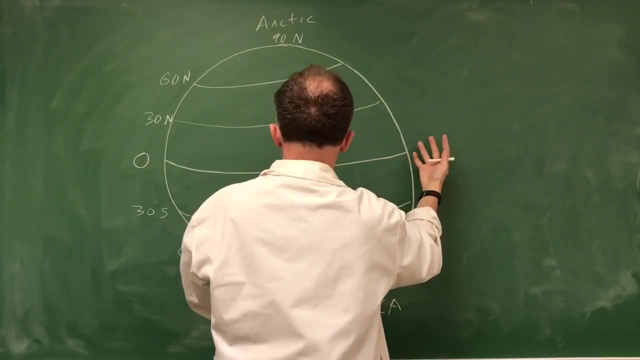 way, because when you get up every morning, the sun rises in the east. So if it's dark here right now and the sun's over there, we have to be spinning this way for the sun to rise in the east. If we were spinning the other way, the sun would rise in the west. So we're spinning. 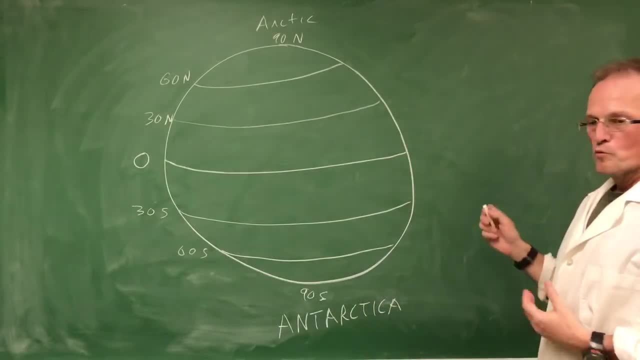 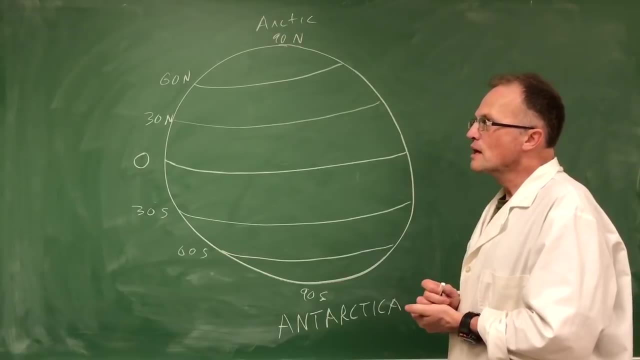 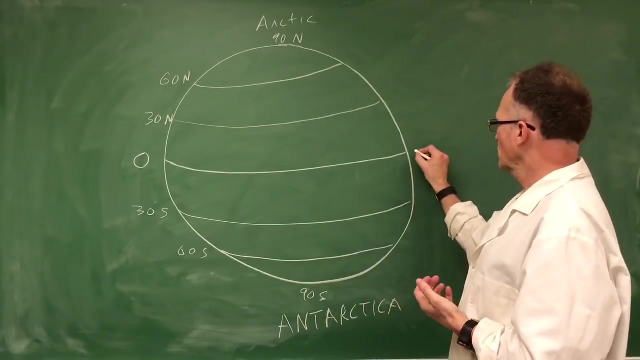 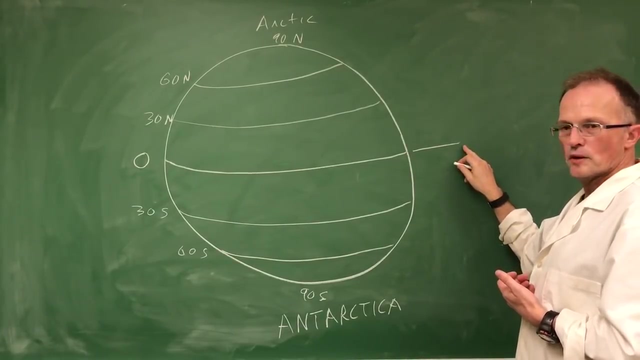 this way. Okay, so the basic principles to generate the circulation of the air is the fact that hot air rises. So the equator is the hottest right, So hot air rises at the equator. It's very hot, so it rises a lot. In fact it goes up to about 17 degrees. So 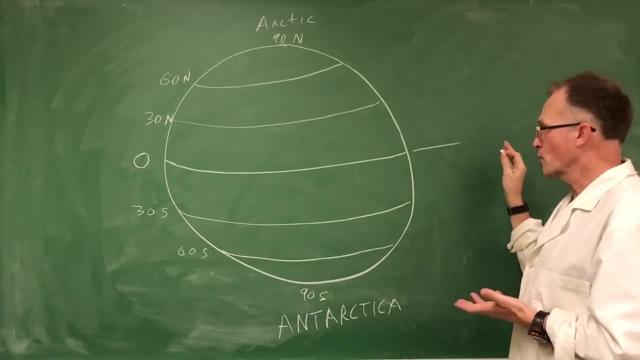 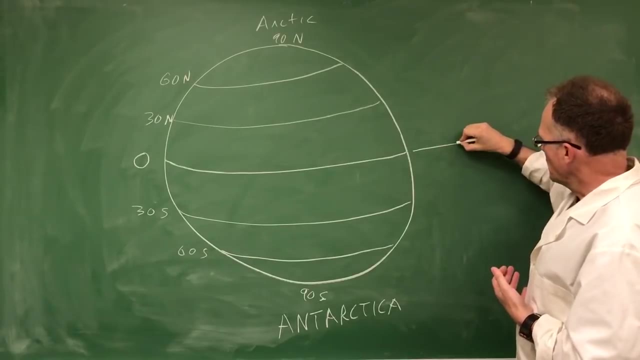 you can see the lower atmosphere, the troposphere, where all the weather happens, about 17 kilometers high at the equator. So then the air has to move. so the air is rising up here, Okay, so it has to move to the north and to the south. So the air moving to the north moves. 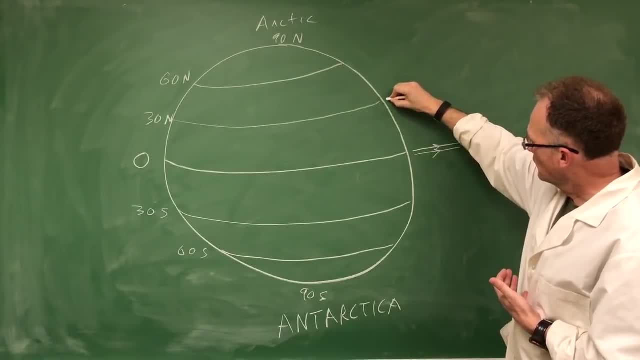 along here and then it descends here and then it retraces here. So this is a convection cell that is generated And we get the air moving to the north and to the south. So this is a convection cell and we get the hot air coming down And we get the air moving up and 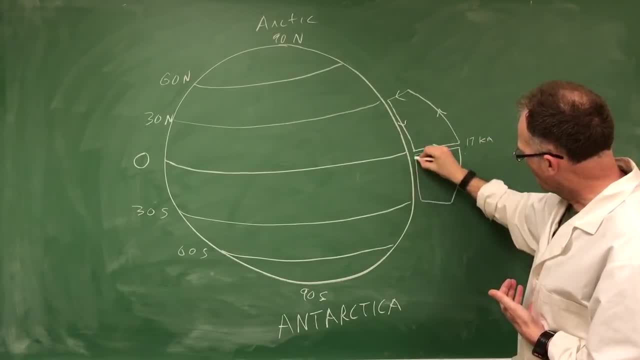 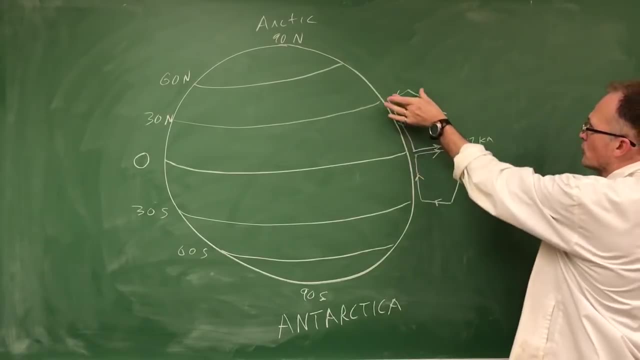 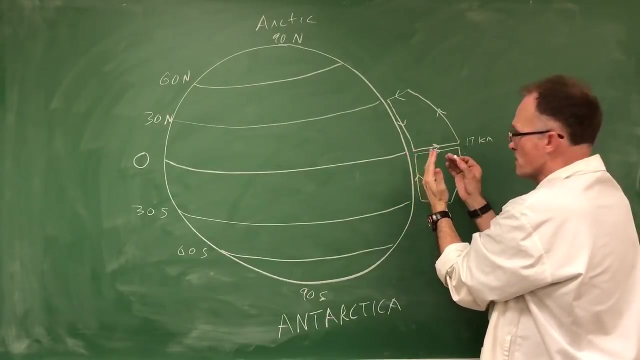 get a similar one in the southern hemisphere. Now, a couple things that you'll notice is: the thickness here is 17 kilometers and it's declining here and it'll decline more and more because cold air is compressed, stays nearer to the surface of the earth, warm air expands and fills more of the of the it makes a. 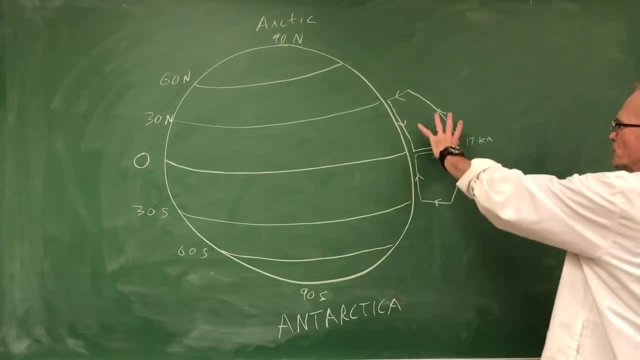 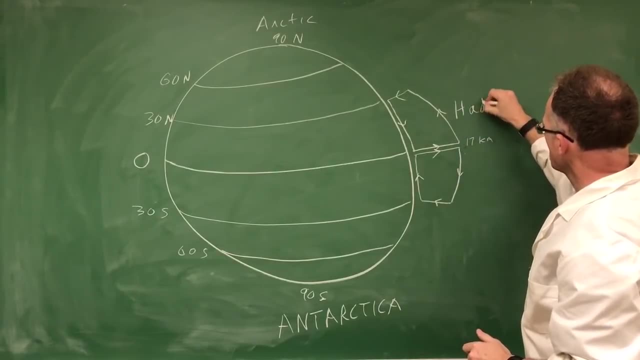 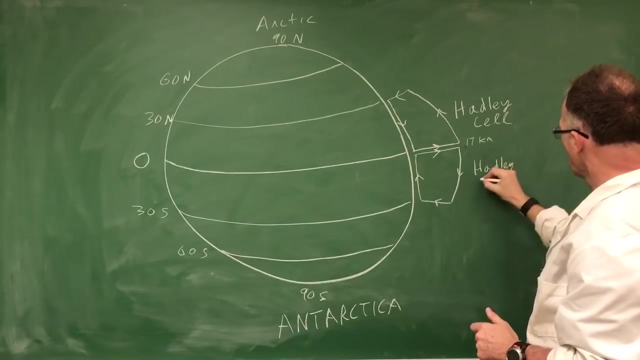 lower atmosphere thicker. Turn this on its side and it's just a convection cell. by the way, these things are called Hadley cells h-a-d-l-e-y. this is the Hadley cell. okay, turn it on its side. let's say we have a kettle of water, okay. 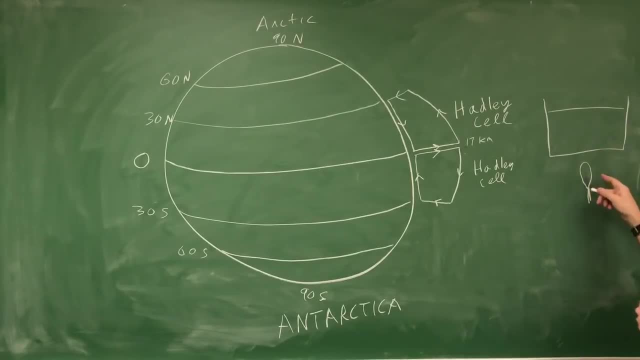 we put. we put it on the burner, so we have flame here, we're heating the water. the water rises directly underneath, goes to the outer cool area and comes back around. it forms a convection cell like this in the water. okay, it rises, comes across, right. so this is the motion: put some pepper in hot. 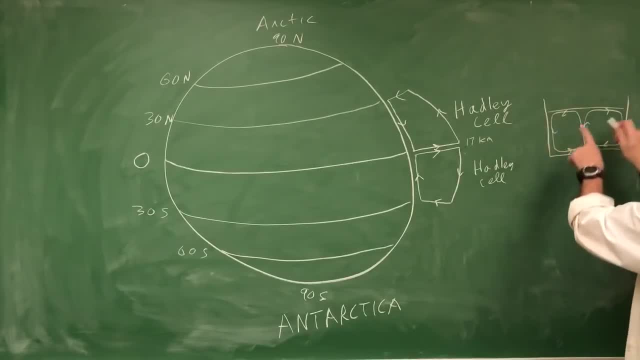 water and boil it just to see this pattern yourself. okay, now of course, it will happen in three dimensions. you'll get this convection cell all the way around to two different cells. I'm drawing it in just two dimensions, okay, so this is exactly what we have. the equator is the hottest. hot air rises. 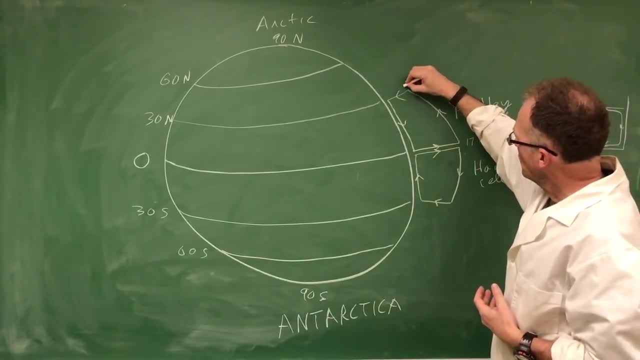 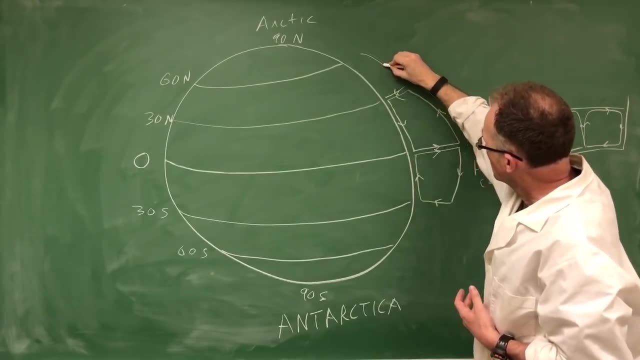 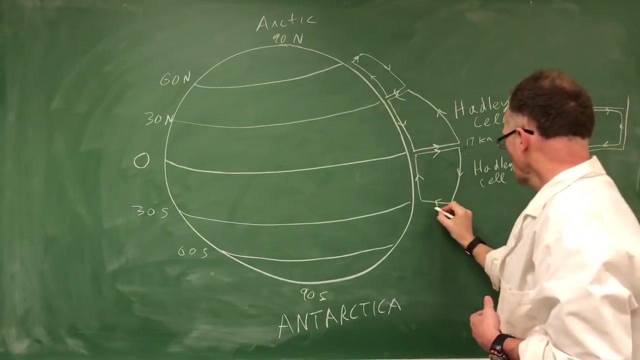 okay, now think of this as a set of gears. so the air here is obviously descending, and it will. it will have to come in from over here and it will have to leave over here and then it will rise up here. so the same thing happens here. okay, the. 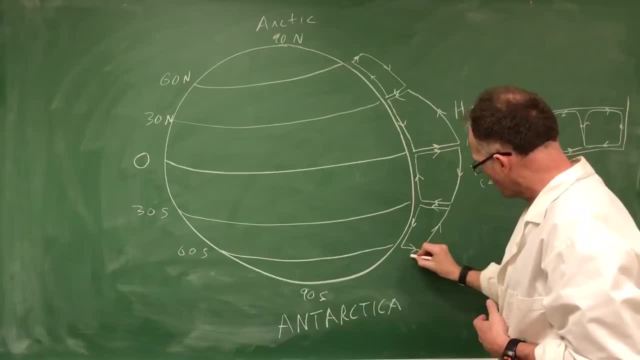 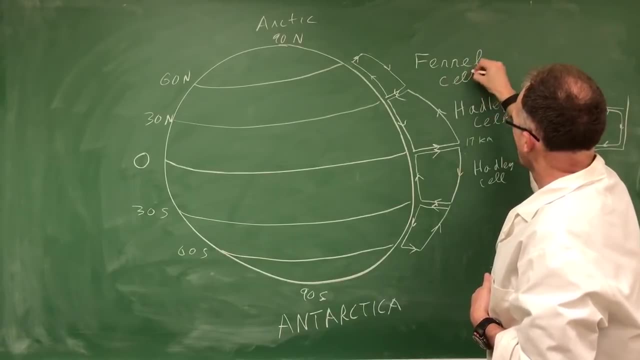 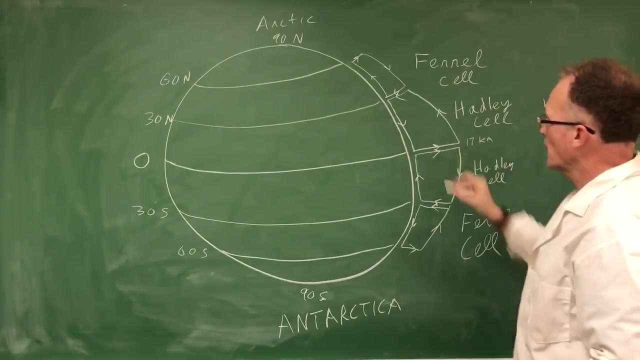 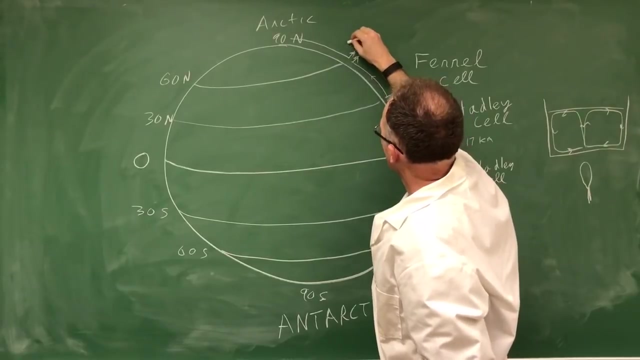 air is coming down. it comes in here, it comes out here, comes up there. okay, this is called the ferrule cell. okay, this is a cross-section pattern. now again you can guess what's going to happen here is: the air comes up here, it has to come from here, it has to go over. 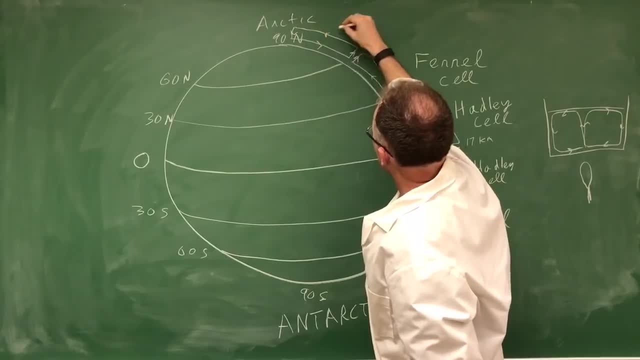 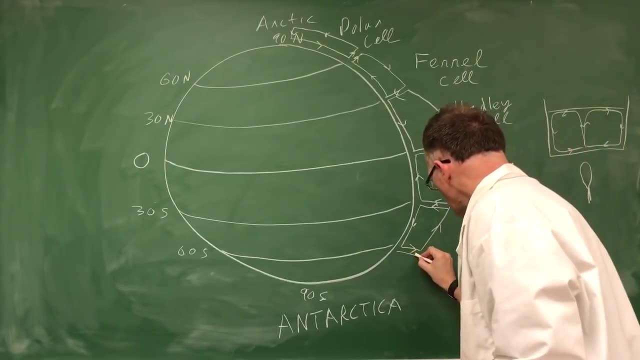 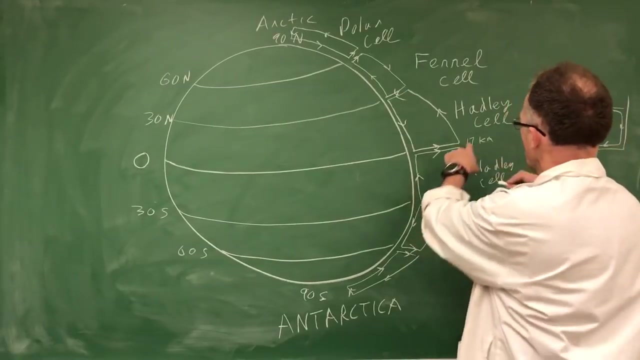 here and descend here. okay, this is a polar cell and we'll draw it over here to rises. here comes this way, comes down, comes down, okay, same thing, okay. so this is what we see for the cross-section. this is 17 kilometers. the air is very cold at the poles. so this sickness of air, if you like, at the pole is only about seven kilometers thick. okay, so seven kilometers, this isn't much really. when you talk about three and a half kilometers of ice on Greenland, you know the bedrock is also elevated. you know the altitude of that ice is well, about three, three kilometers. 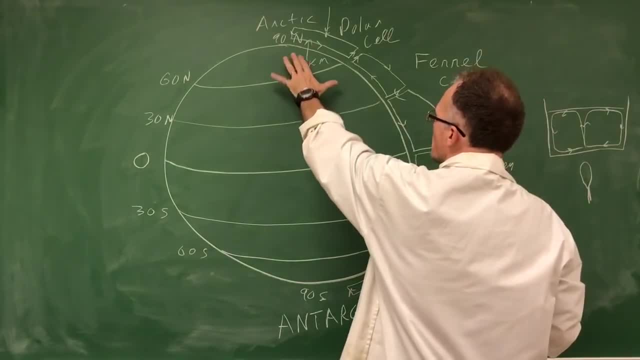 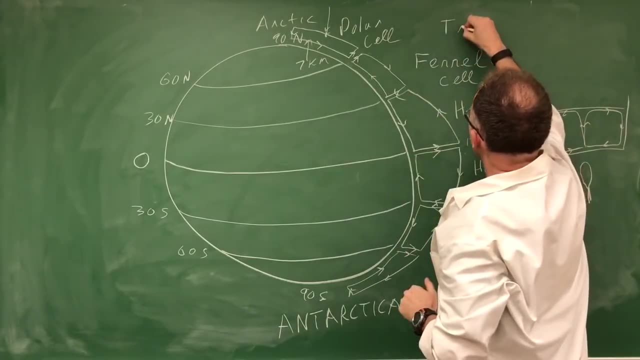 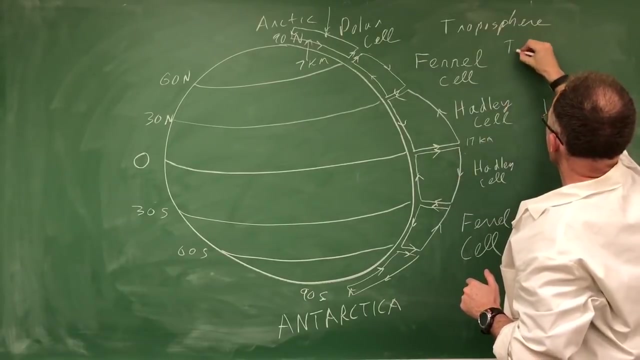 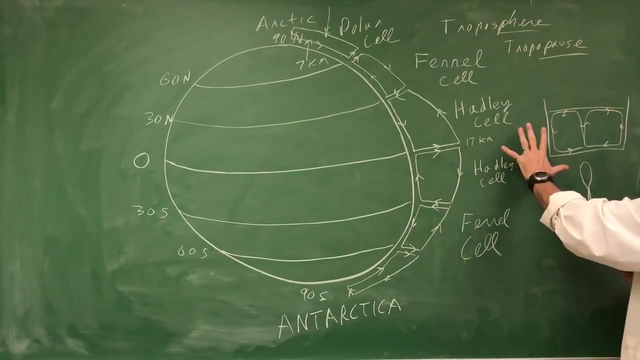 anyway, then three and a half kilometers, it's almost halfway up to the, to the top of the tropopause. so this is the tropopause, the troposphere, rather troposphere, and the upper edge of the troposphere is the tropopause, and then above it is the stratosphere. 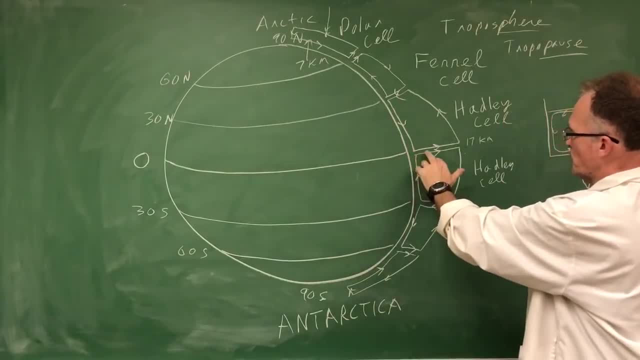 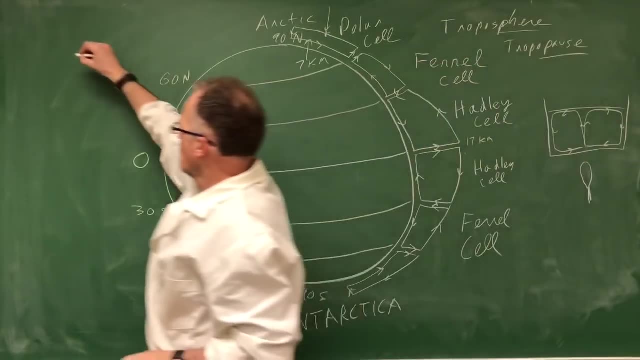 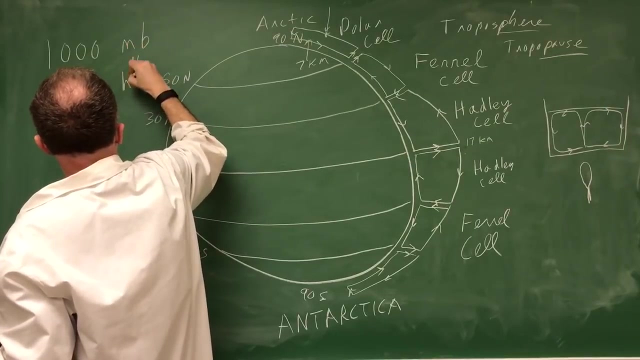 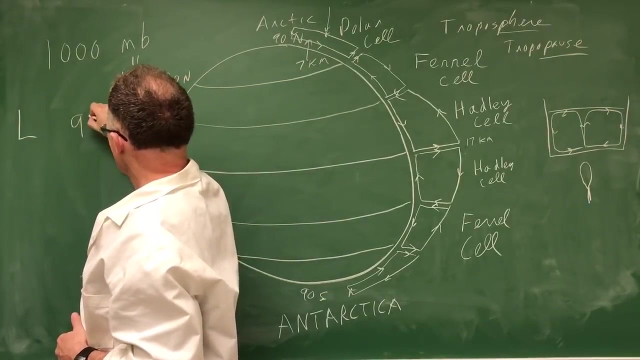 okay, so what does this do on the surface of the earth? the air is rising here now. the pressure on the surface of the earth is typically about a thousand millivar, which the millivar is equal to a hexapascal. you'll see both units okay. a low-pressure area will be maybe 980 or something. at the surface, a high 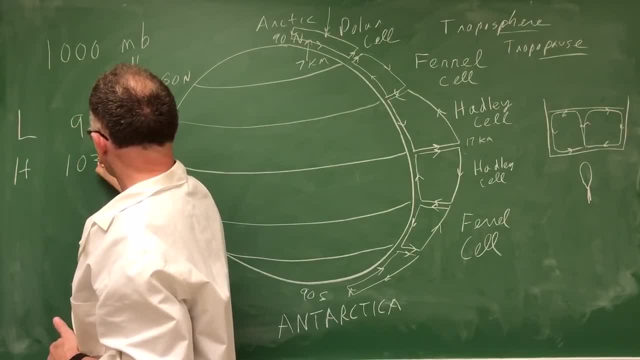 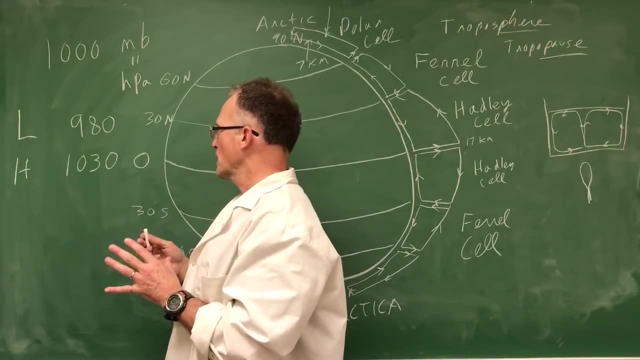 pressure area will be to be 1020 or 1040 or something like that. so this is the surface of the earth. it's very low pressure. okay, we're going to draw in the 30, Okay, so if you go across North America, the highs and lows typically vary. 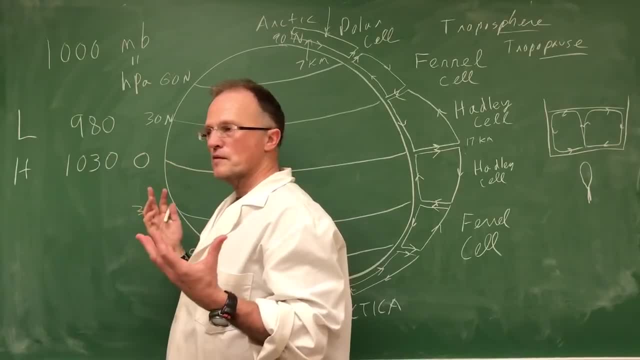 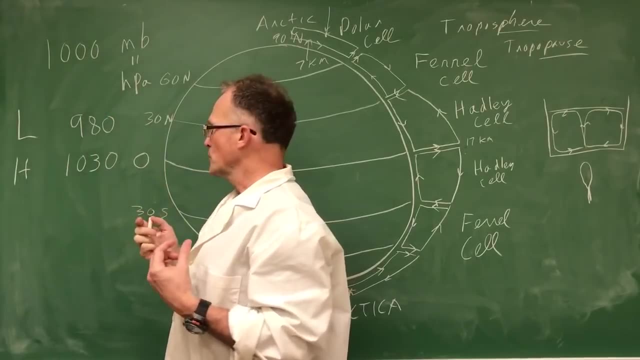 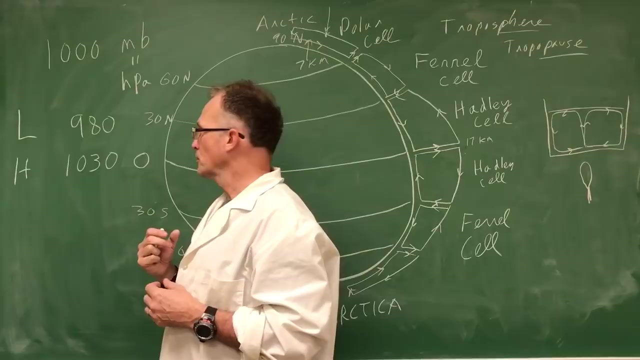 In slightly in this range or slightly less this range. They typically vary only about 30 millibar, So maybe plus or minus 15 millibar above the nominal. Typically, when you get a tropical, when you get a tornado, It's very, very low pressure in the in the eye of the tornado, the center of the tornado. if you get a hurricane, 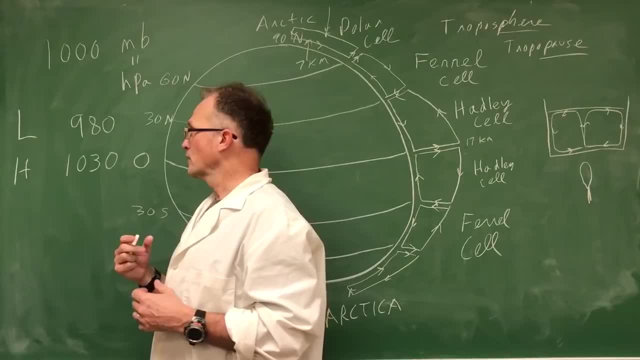 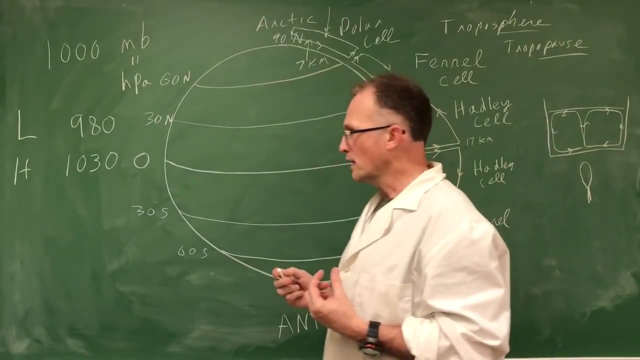 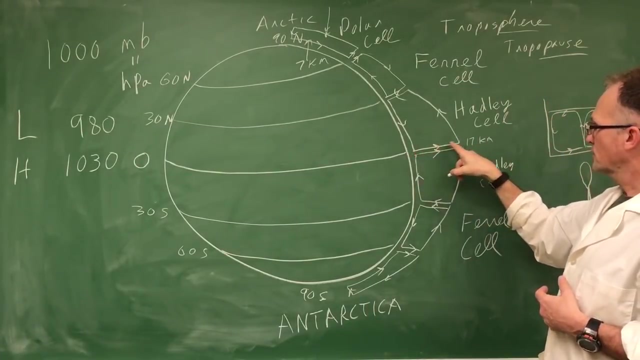 Then it's very, very low pressure inside a hurricane. So so any lows are associated with storms. highs are associated with With very hot weather, no clouds. Why is that? Okay, so the air is very humid at the equator. It's rising up. as you rise up, the air cools, the water vapor condenses into clouds. 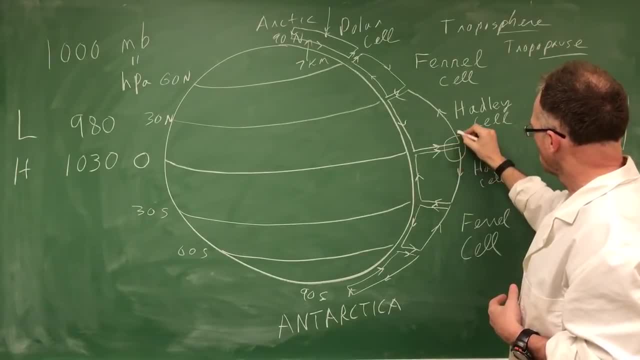 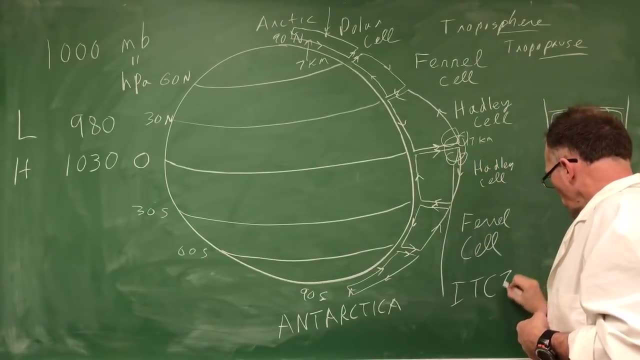 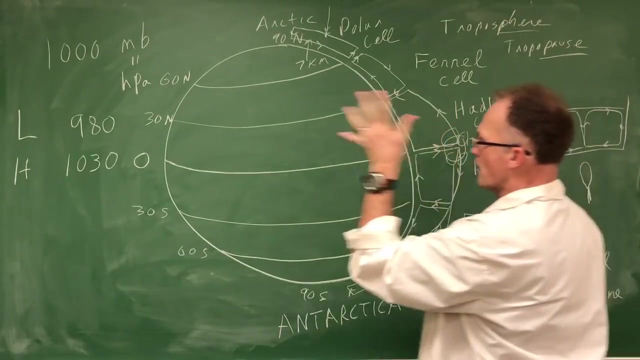 So we get a band of clouds at the equator. We get a band of clouds here. this is called the ITCZ or intertropical, Intertropical Convergent Zone. so this band of clouds will go around the planet. Now it's not exactly at the equator. 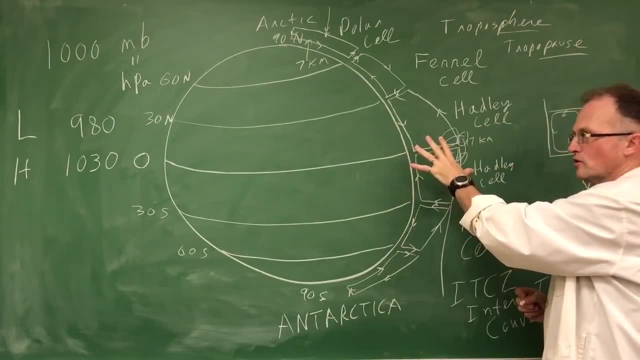 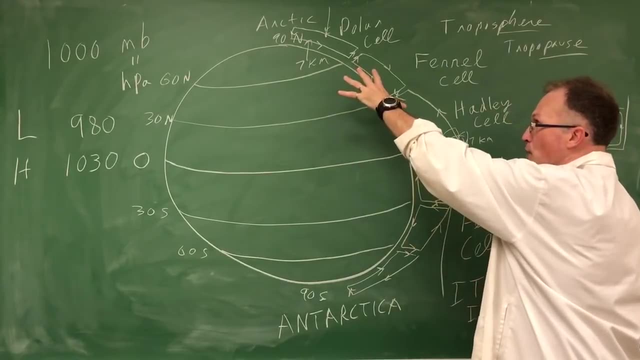 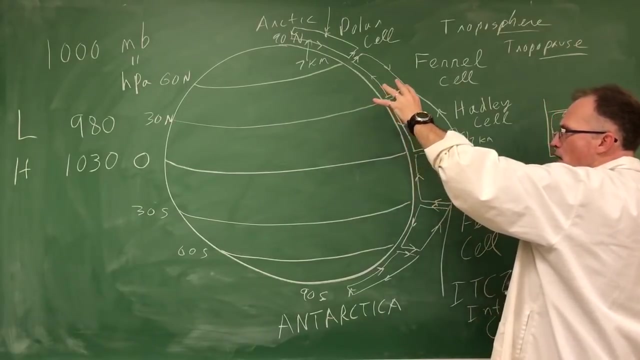 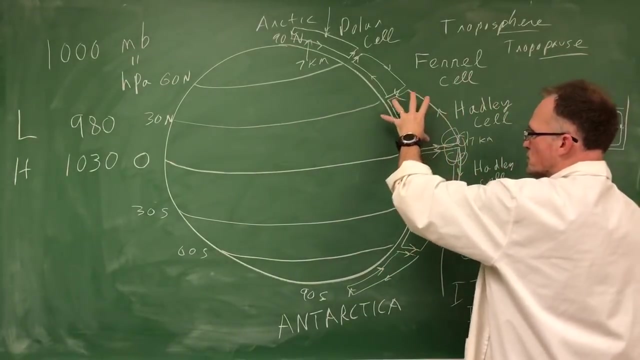 If the Sun is over the equator at the equinoxes, it will be close to the equator when the Sun's in the Boreal summer, so the Northern Hemisphere summer. then they saw the Basically the temperature, The equilibrium temperature line, if you like, will be shifted north. the ITCZ will be shifted north and in. 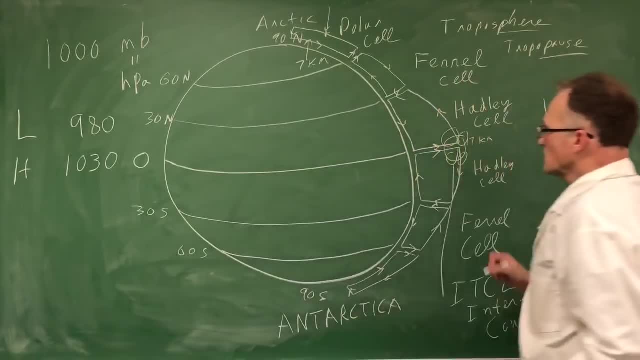 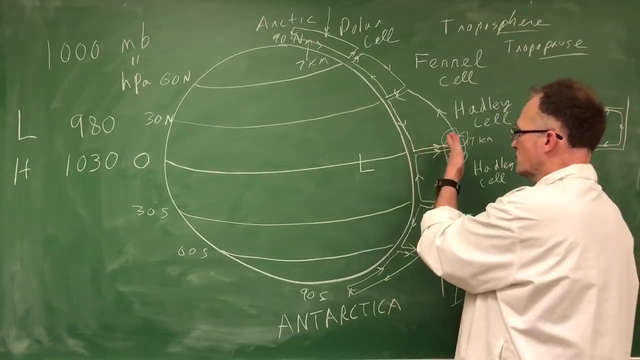 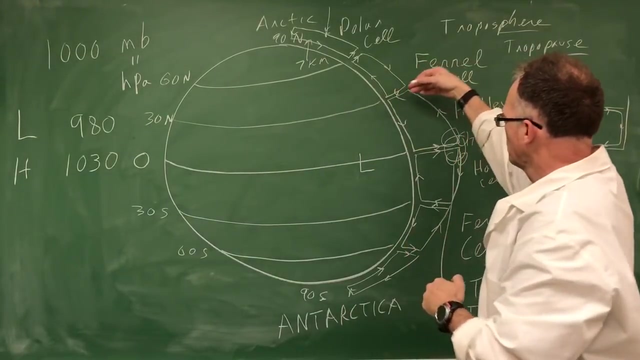 Opposite. in the northern winter it was shifted to the south. So what happens when air rises at the surface? it creates a low pressure area at the surface. right the air rises. something has to Fill it. air rushes in lower pressure at the surface. Okay, air is coming down here. 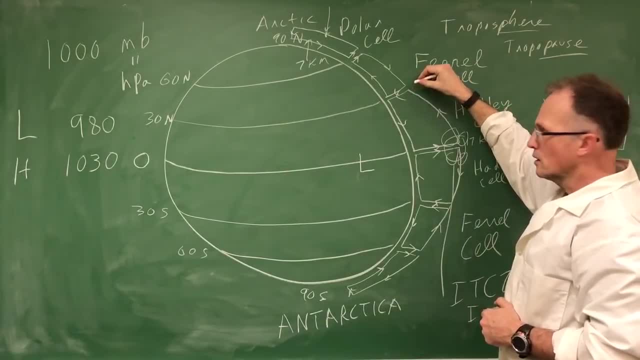 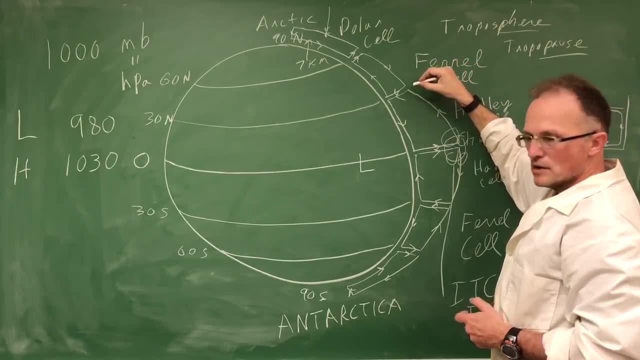 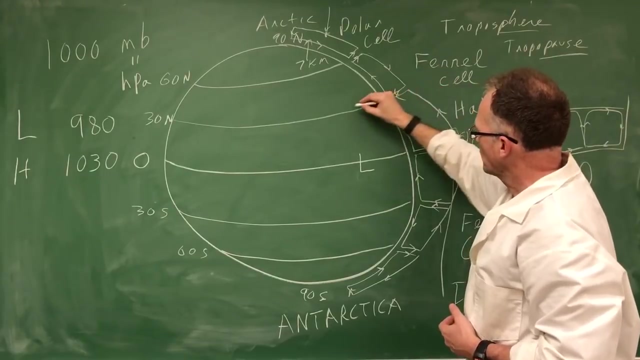 The air has lost all its moisture because hot air, you know. the air is very cold up aloft, So the moisture has already come out and condensed into water droplets, clouds, Perhaps even rained out. So the air is very dry. that's coming down there, So it's pushing against the ground. It creates a high pressure here. 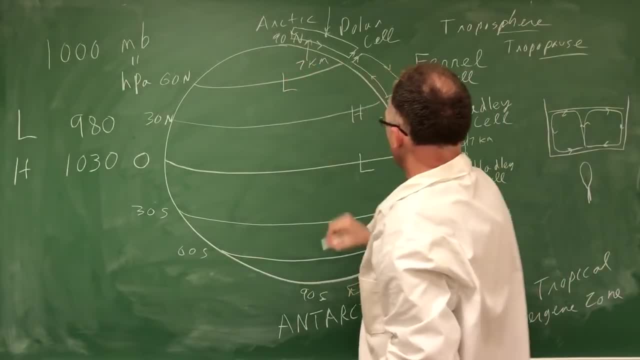 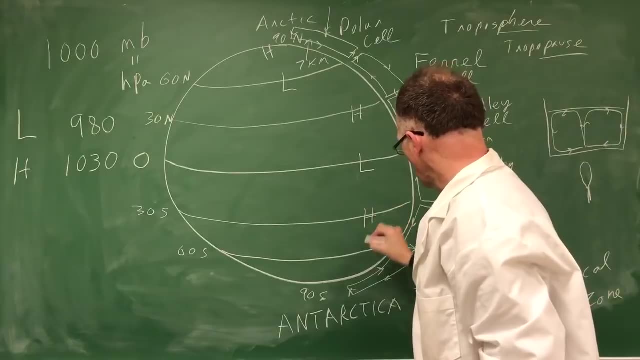 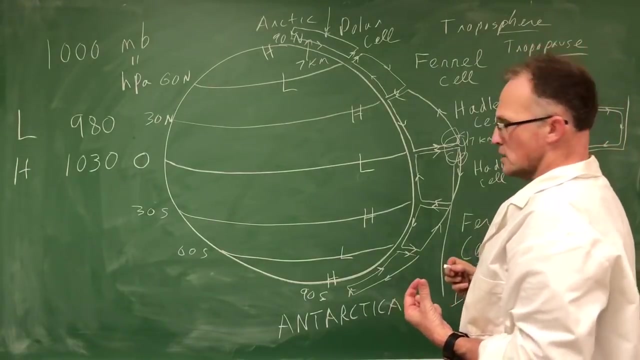 Air is rising here creates a low pressure at the surface, and Air is descending at the pole, creating a high pressure there. Okay, so this alternates down here: high, low and high for the same reason. Okay, So now the other thing that you need to know is about the Coriolis force. We said that the earth is spinning this way. 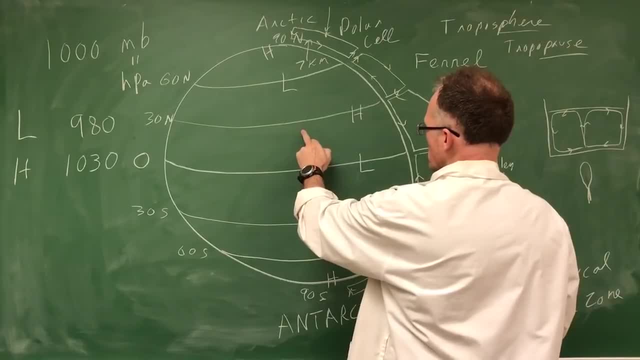 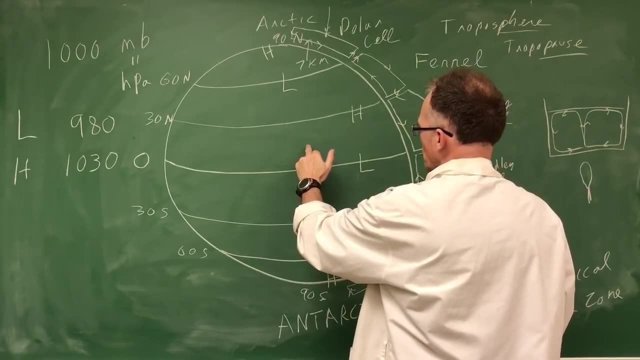 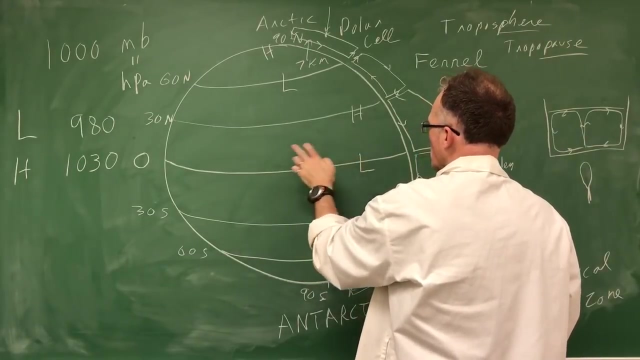 So if you're here and you start moving in this direction- Here you're moving to this way very quickly- as you go up here, the Earth's surface- Because you're the radius to the center of rotation- is decreasing. the earth will be moving slower here and to the this way here. so the, the, 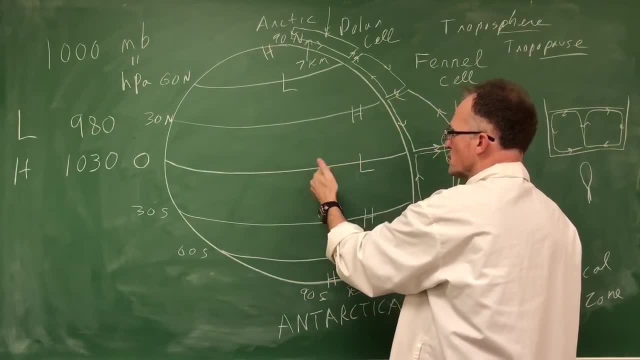 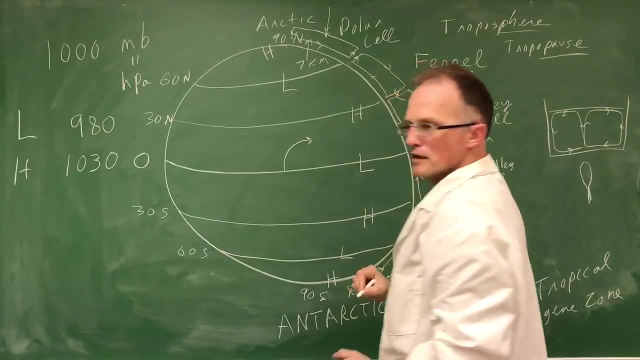 Velocity on the surface is highest here to this direction, So it still has that component. So as you move up here, basically this causes a deflection to the right in the northern hemisphere. You always get a deflection of objects. It doesn't affect the speed, It just changes the direction. 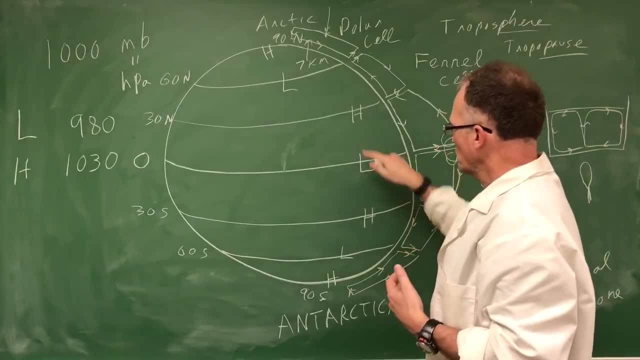 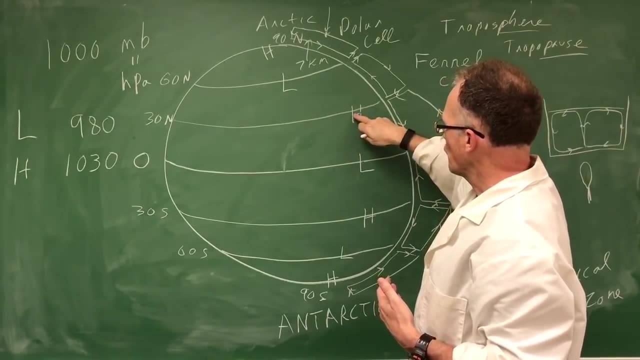 Okay, but in this case this is high pressure, This is low pressure. So air wants to go from high to low pressure. Okay, air wants to go from high to low pressure. So here to here it deflects to the right in the northern hemisphere. 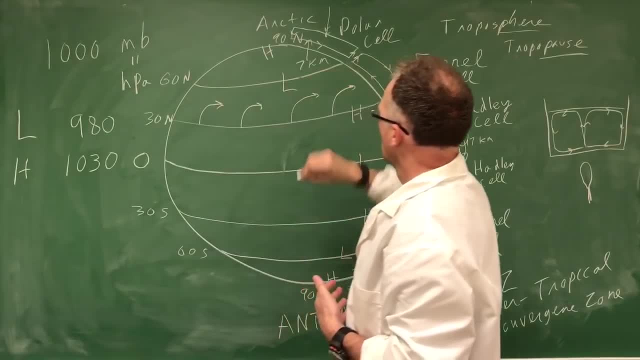 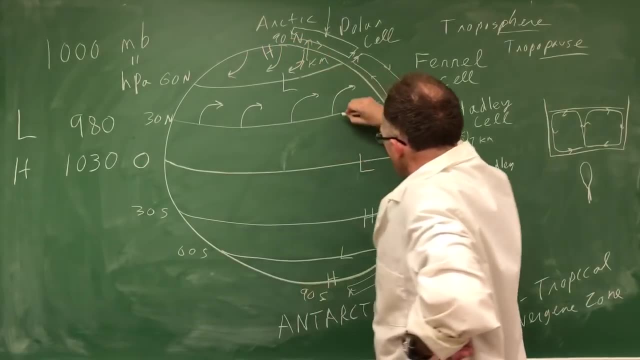 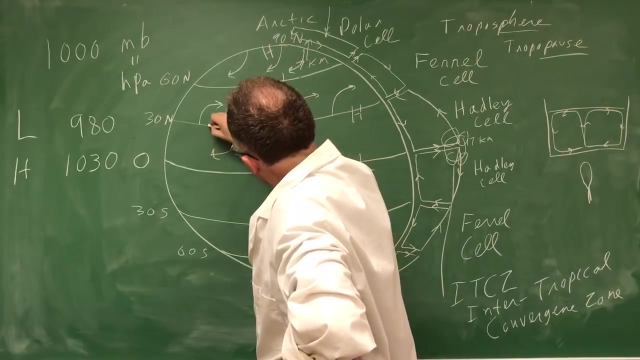 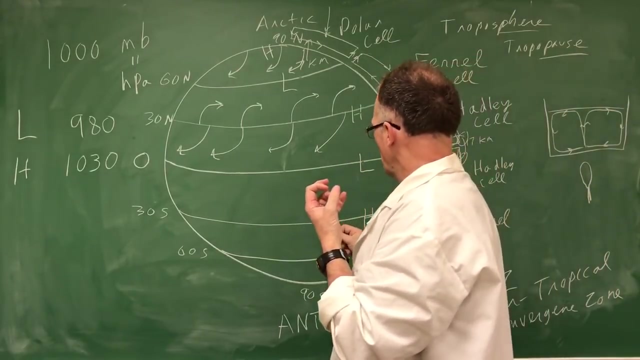 From the Coriolis force. Okay. from high to low pressure, it deflects to the right. From high to low pressure, It deflects to the right. put yourself upside down. it deflects to the right. Okay now, in the southern hemisphere it's opposite. The Coriolis force makes things deflect to the left. So, high to low, we get a deflection to the left. 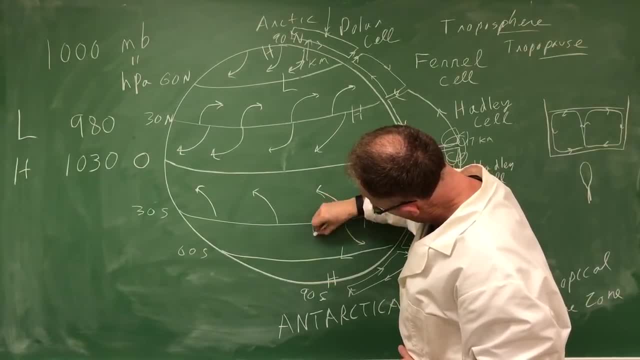 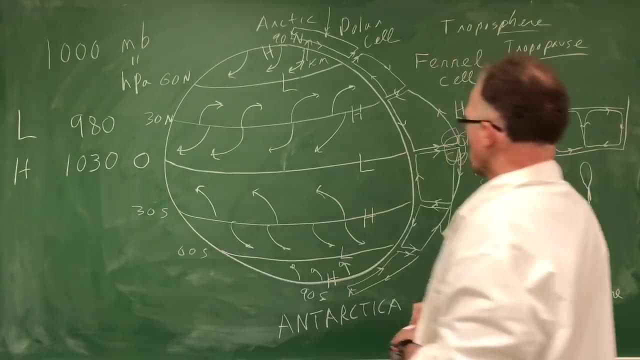 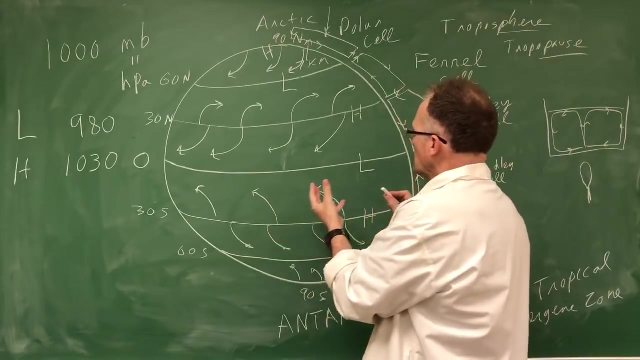 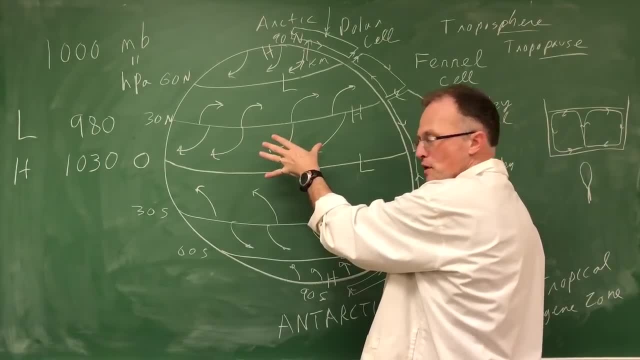 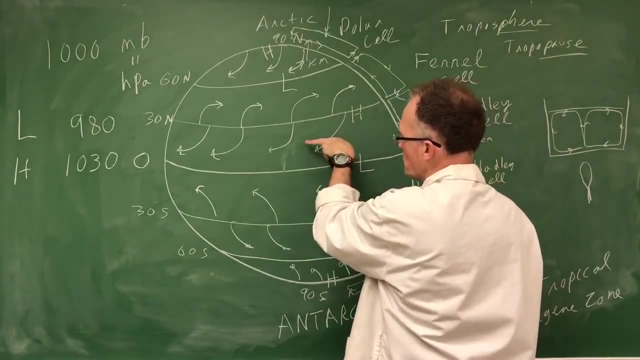 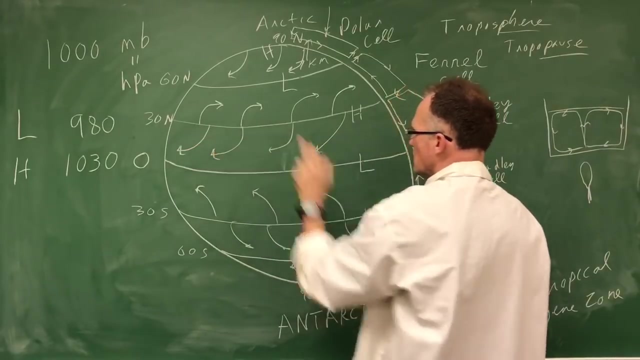 and low pressure area. there is no friction with the earth. The boundary layer is about 1.5 kilometers, so you get geostrophic flow. So the flow of the air would be parallel to the isobar lines. This is a low pressure line. high pressure line. be in this direction. Now, at the surface it doesn't. 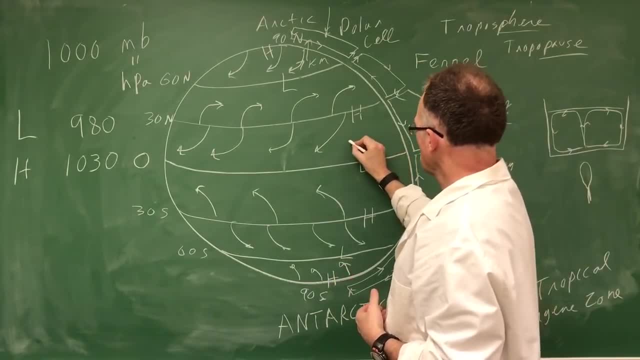 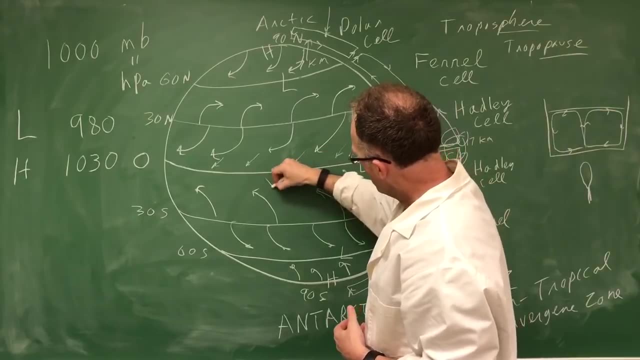 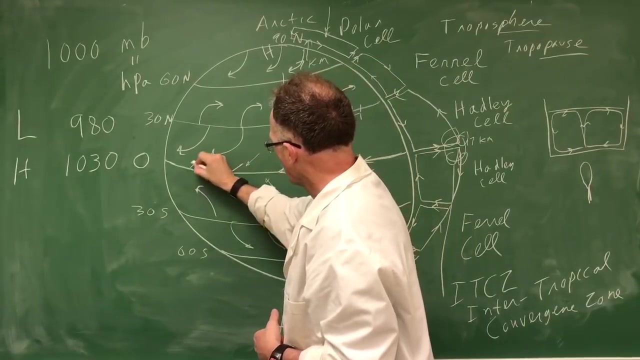 bend all the way. It's not geostrophic because of the friction, So you tend to get the air moving like this. at lines to the isobar We'll get air moving this way, So this generates the trade winds. The air motion at the equator is this direction. The trade winds are moving here. 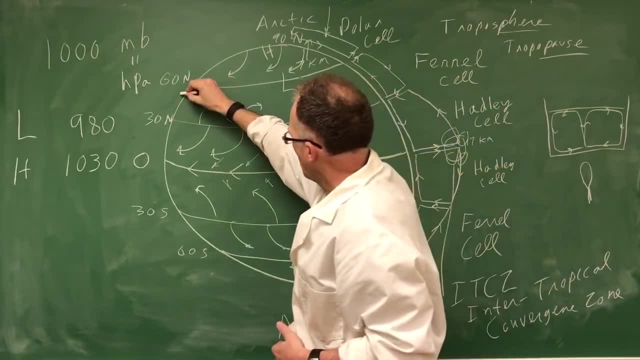 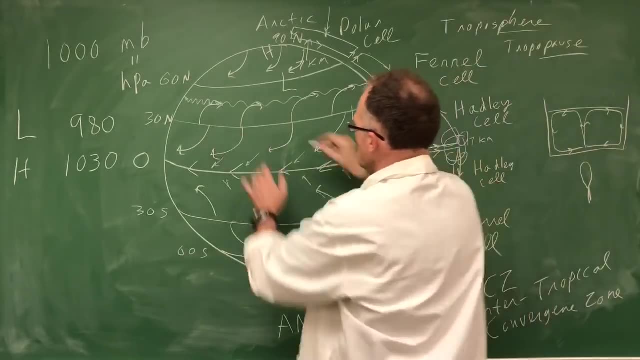 Up here where the jet streams are. okay, this is where the jet stream is right. It's not that wavy, I'm just illustrating. So the jet stream is moving basically zonally west to east in this direction. 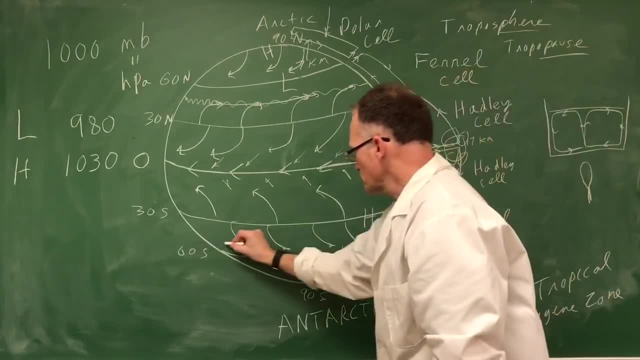 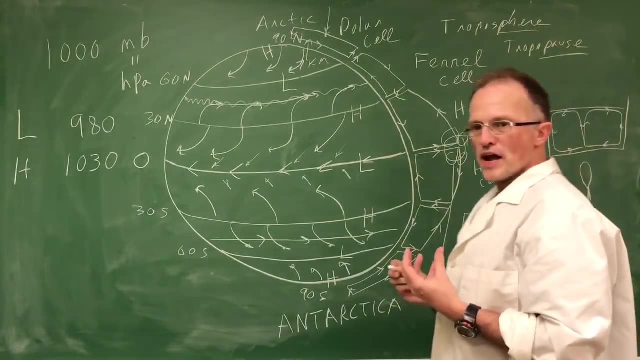 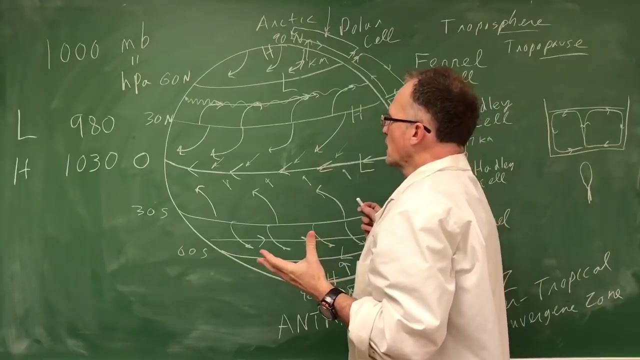 Notice, at 45 degrees south. the jet stream is also moving this way, which is west to east. Okay, now there's other factors that are coming into play. So there's mountains, There's mountains, There's land-ocean contrast, And there's a tendency for the jet stream to reach. 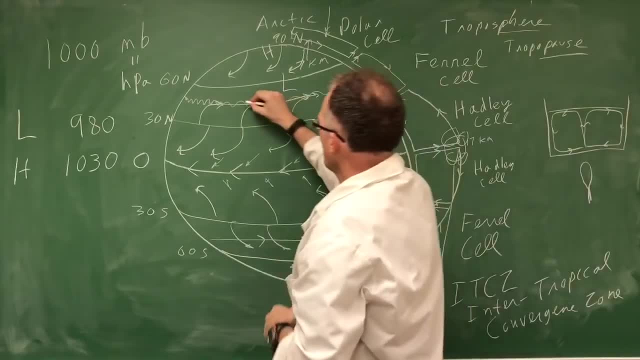 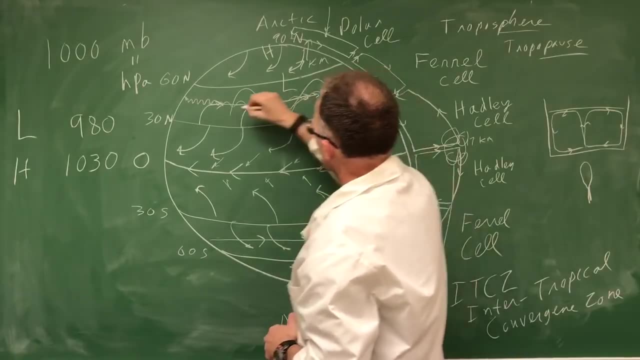 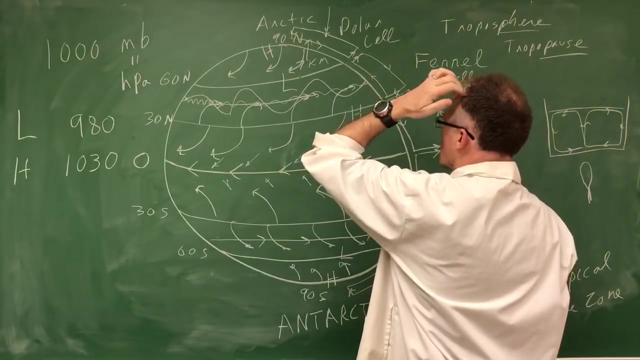 a resonance with three wavelengths, So this is a wavelength of the jet stream. here The jet stream in actuality will look like this: going around the surface, going around the earth, rather at the height of the, of the up near the tropopause.